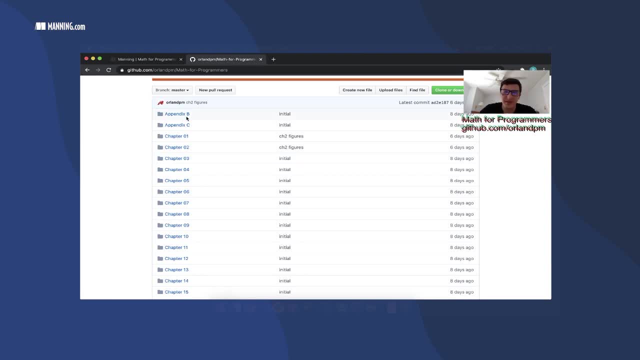 not to do anything directly out of the book. Instead, I wanted to kind of show something that was using some of the concepts from the book but doing a kind of new application that isn't directly covered in the book. So what I'm going to be covering is a mathematical 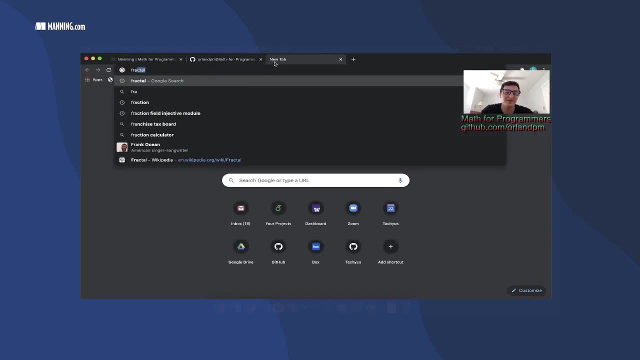 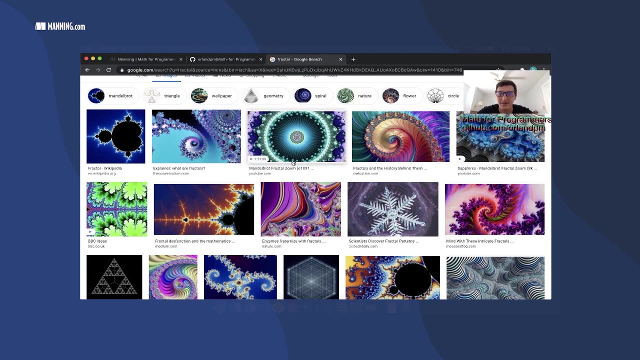 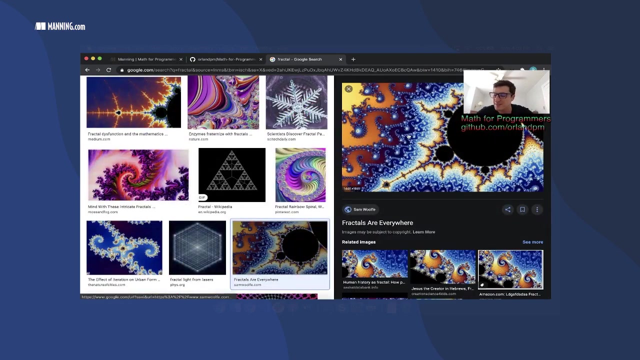 concept called fractals and fractals. if you just search for fractal, you can find a bunch of cool pictures of what a fractal is. Fractals are these kind of weird, complex geometric things. so if you there's some that are recognizable. this is the Mandelbrot set. this is a. 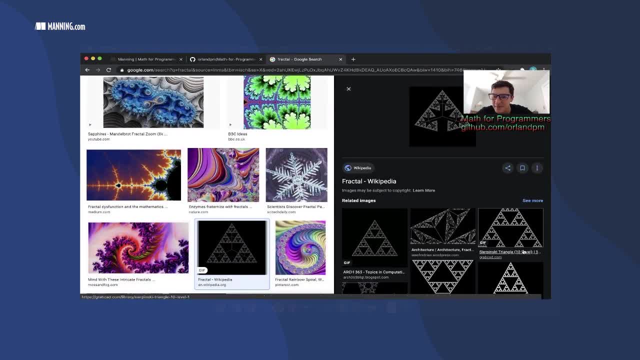 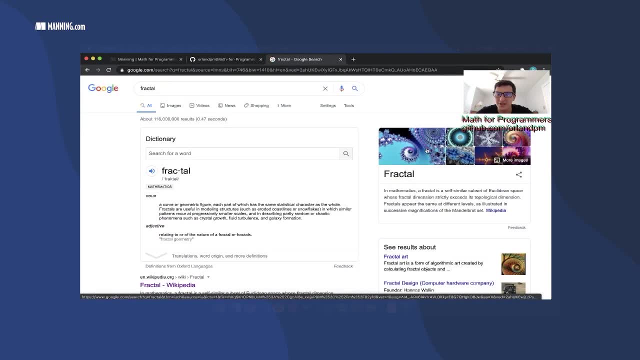 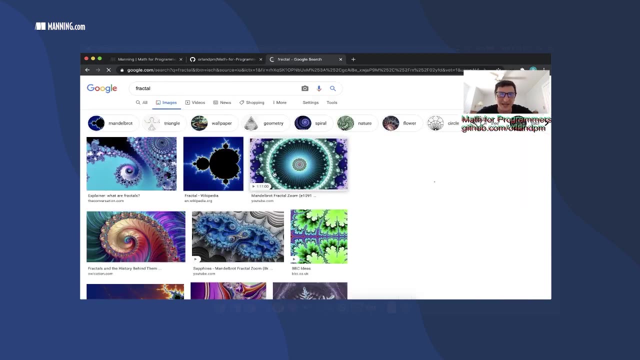 special fractal. this is the Sierpinski triangle, if I'm not mistaken, So you can find a bunch of these online if you search, and they're all. they're all cool to look at. There's a lot of math that underlies these, these fractal graphics, and it's actually despite how complicated these. 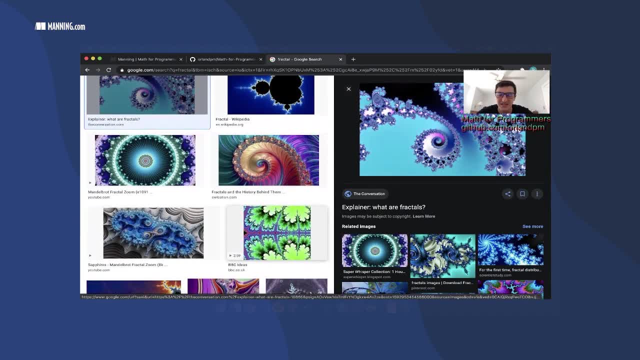 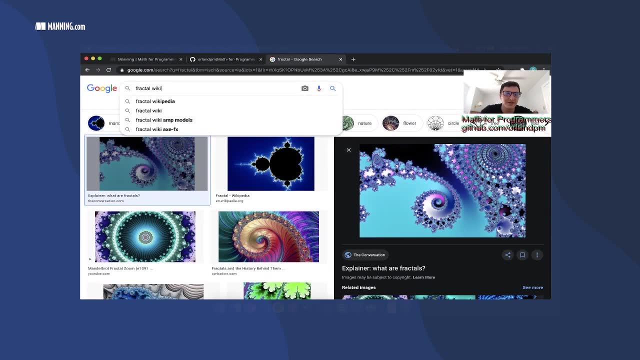 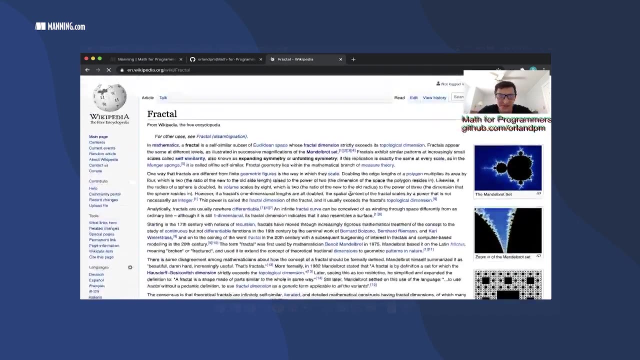 look relative to some of the geometric things you may have seen in in the math class. they're actually pretty simple to define. So I guess probably the simplest thing to do is to show you what a fractal is. So if you go to Wikipedia, I'm sure they have a list of fractals here. 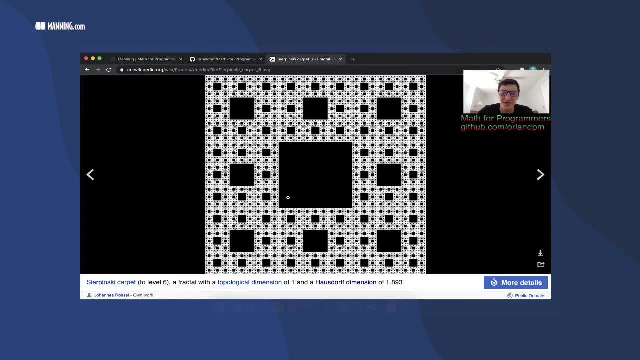 Let's see. here's one that's called the Sierpinski carpet. This is a good example of a fractal, because it shows you that one of the key properties of a fractal is that it's self-similar. So in the middle here of the fractal you have this black square, and then basically what? 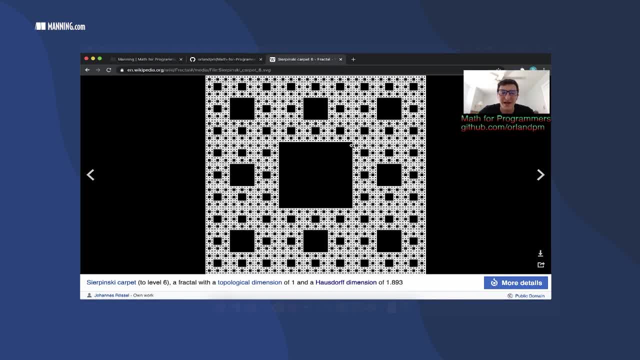 the fractal is defined at is this black square in the middle, and then there are eight copies of the fractal around the outside, So each if you look at any of these eight kind of boxes around the edge, you'll see that each of them has a black square in the middle and then there are eight more copies around. 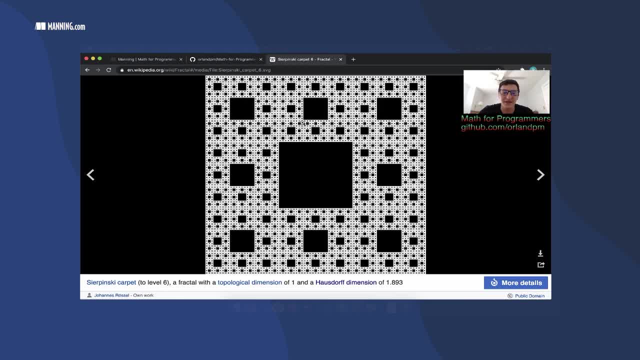 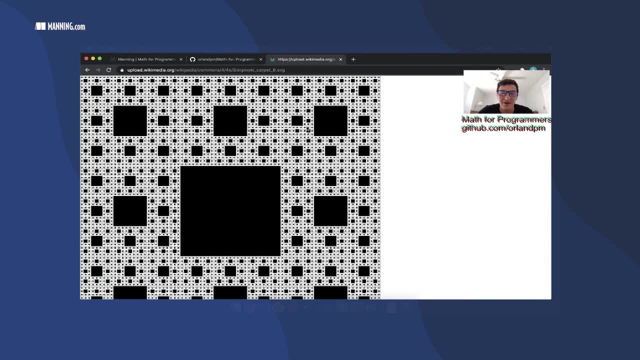 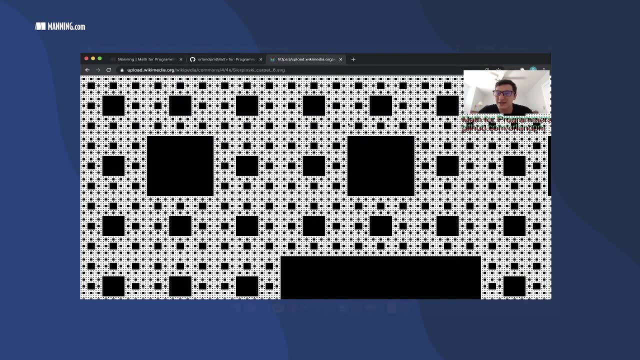 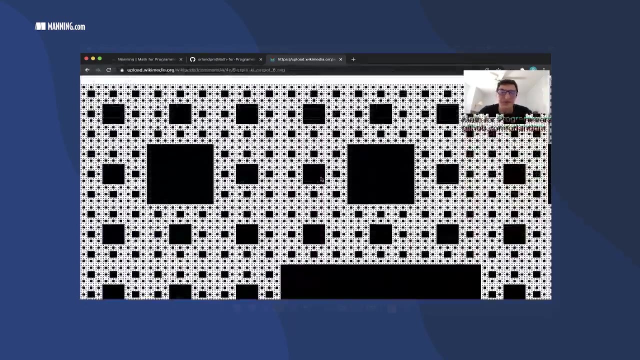 the edge, that look like the whole, like the whole figure. So if you zoom in, you continue to see. no matter how far you zoom, you'll just see more and more shapes that are kind of like, identical to the appearance of the fractal. What we'll do today, in the next hour or so, is I'll use some of the concepts from the book math for programmers and we'll generate some cool kind of self-similar shapes like this and then talk a little bit more about the concept of fractals and what they are. 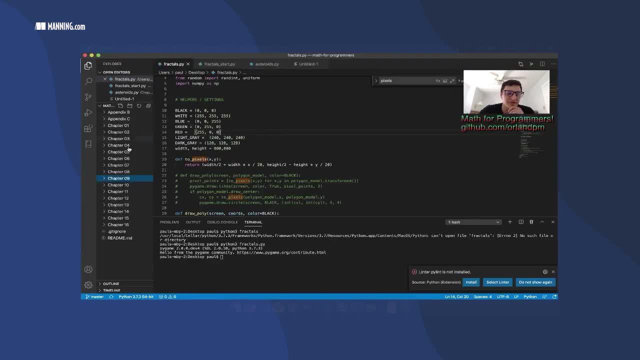 If you've got the source code downloaded for math for programmers and we won't use it directly, but I just wanted to show you guys where it is. for context, Like I said, it's organized by chapter. most of the chapters have a Jupyter notebook, which is I should. I should say, first of all, all of the code for math for programmers is done in Python, and Python is one of the best languages to use if you're learning math and especially if you're, if you're doing math and code. 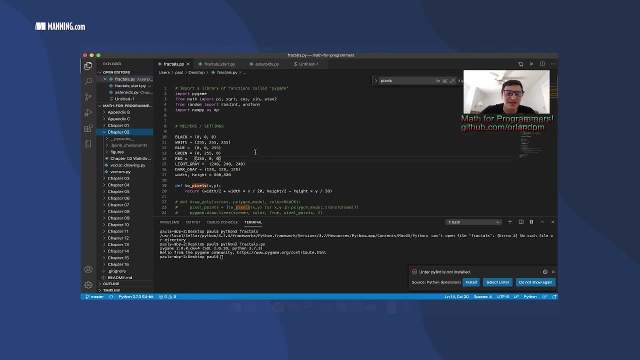 There are a couple reasons for that. First of all, Python is very. it's a simple language and it's widely used. Second of all, it's got a lot of good libraries for numerical and mathematical computations, So it's kind of the de facto standard for data science and and for machine learning. 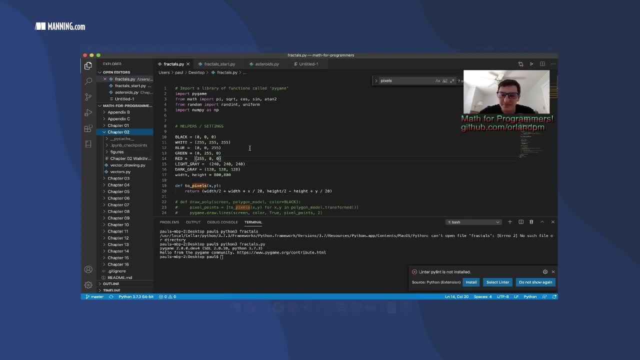 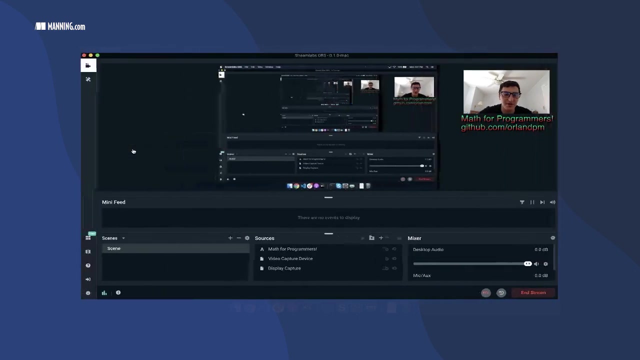 So further within Python, there's this tool called Jupyter, which is a way of kind of having a more visual version of a interactive session. like you know, you can obviously type Python commands into an interactive session, like many scripting languages, But you can also show you an example here in the source code. 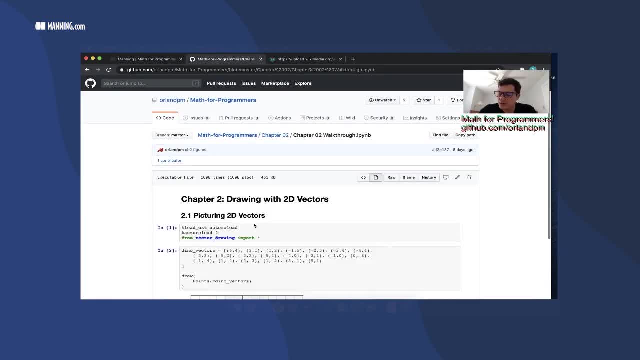 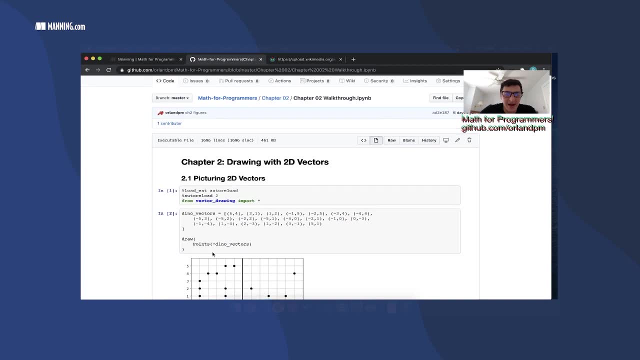 You can also put together a notebook, and what a Jupyter notebook looks like Is the following: so it's kind of like you type code into a box and then, when you execute it, you could get output that's either text like would come out in your command line, or you can get a picture like this: 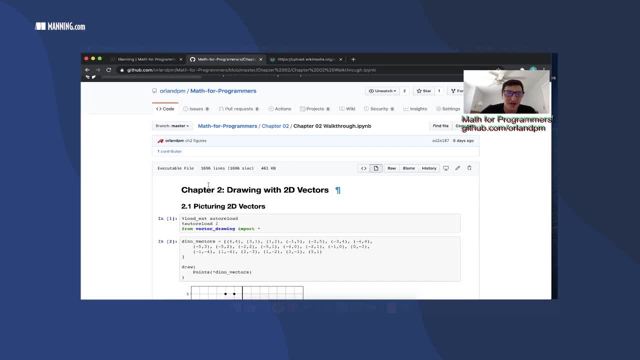 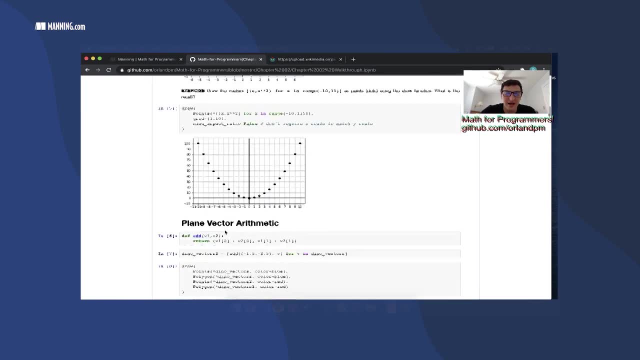 This is the graphic generated by this code. So Jupyter is such a common technology and a way for organizing code that actually when you put a Jupyter notebook on GitHub you can see the whole kind of session drawn out here. I really like this for the for the book math for programmers. 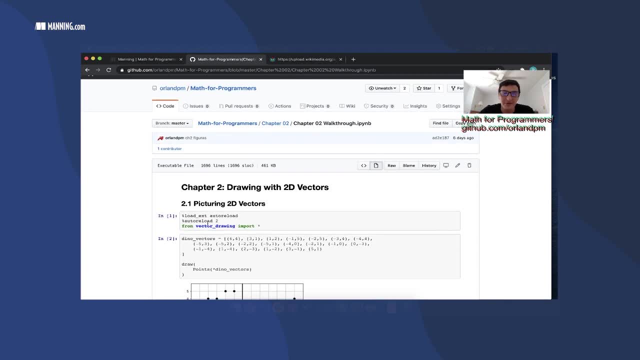 Because it gives you a kind of reproducible way to go through all of the code from the chapter. Otherwise it's kind of hard because you know you see a line of code in the book, but then how do you kind of put it together into a working example? 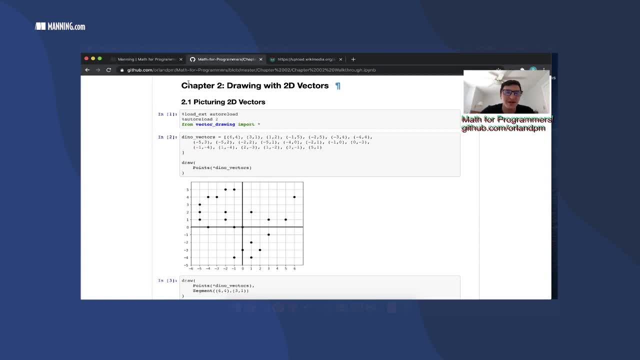 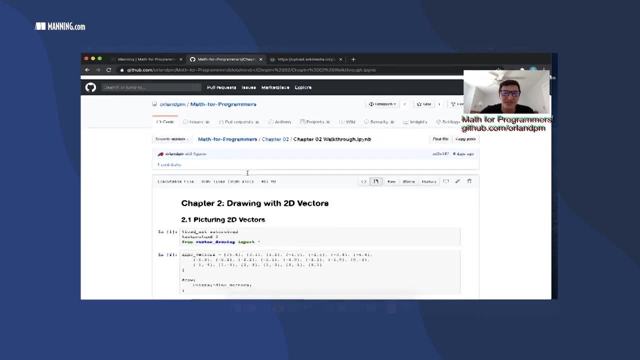 So I hope that if you guys download this and you have all the prerequisites set up which are detailed in the appendix for math for programmers, that you can kind of just run this end to end and work through all of the examples And I hope that that make this makes this book approachable. 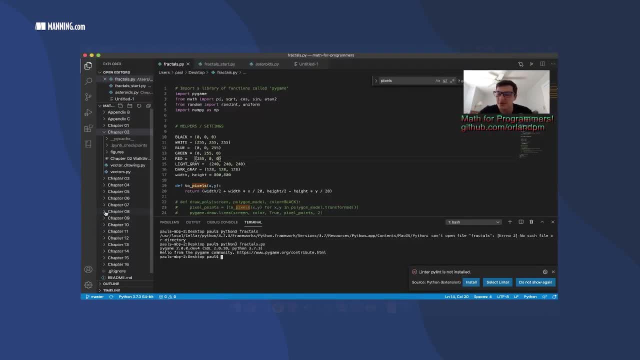 So in some chapters that's not the case And there's some things that you can't do in a Jupyter session. Like you want to have. something that's that's interactive or a real time is not convenient and maybe possible, but it's not convenient to have it in the Jupyter notebook. 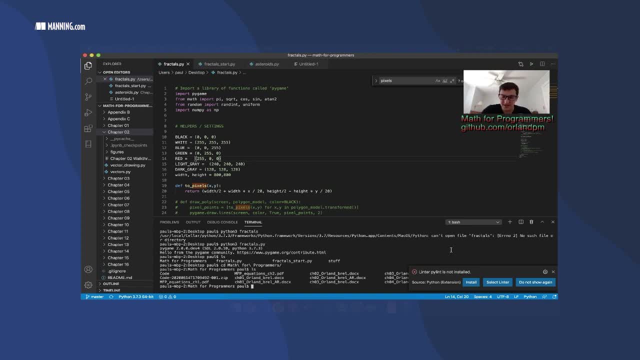 I can show you an example of that, And I think it's chapter Old folder. Okay, let's try chapter nine. So in chapter nine we use an algorithm to do simulation based on physics equations, called Euler's method. And if you do chapter nine, then you will end up building a little video game. 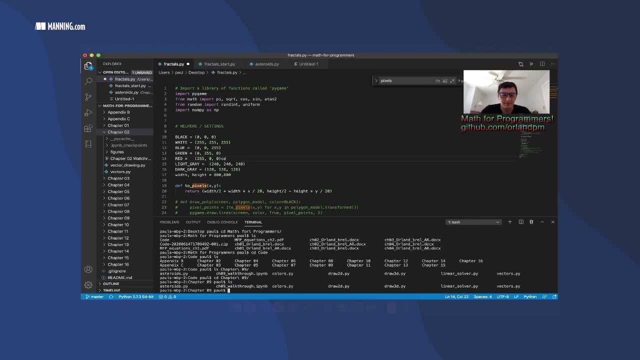 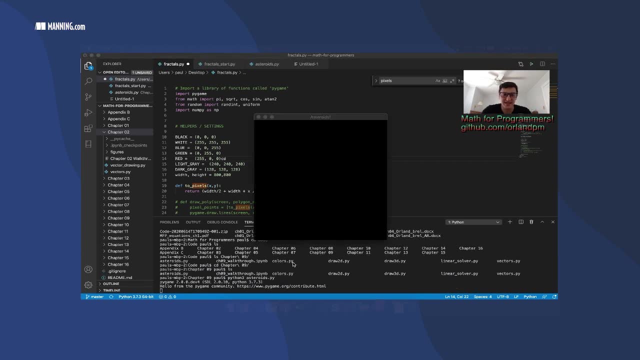 Go to that folder first And you guys have probably seen this type of video game before. It's pretty famous. So this is like an asteroid game, where you have a little spaceship and then there's some asteroids and then you can shoot them and you try and avoid them. 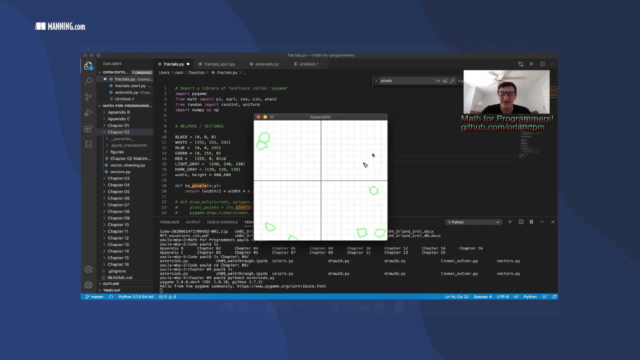 So this, this takes, you know, takes some math of deciding where, in this kind of grid, you're going to draw each of these polygons and how you're going to make them move and how you're going to make them rotate. So that's covered in the book. 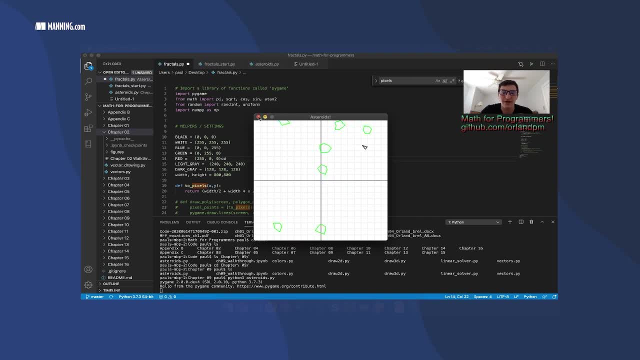 But I'll use this as the starting point For for what we're doing today with fractals. So if you want to, if you want to kind of review the math to get ready for this coding session, you can look at chapter nine and that'll show you how to kind of make the animations that will do and handle the key presses. 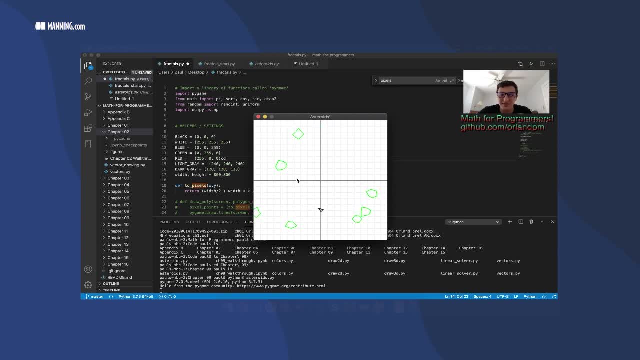 You guys can't see it right now, but I'm I'm pressing on my keyboard to steer the ship and actually, chapter seven and chapter nine will show you how to make the asteroids game, And then chapter two will kind of fill in some of the more basic concepts. 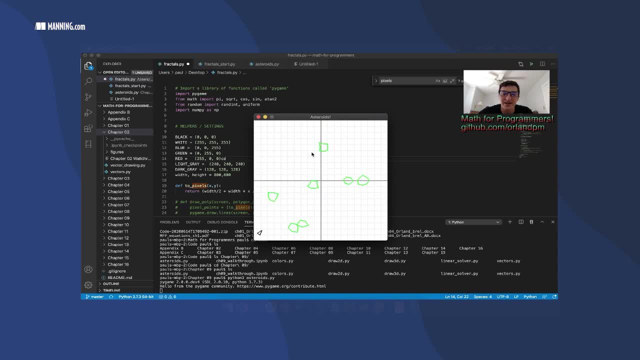 So how do you represent polygons and how do you, you know, how do you use the points in the coordinate plane? I'll kind of go over that as we go today, But that's that's kind of to catch you up on where we're going to start. 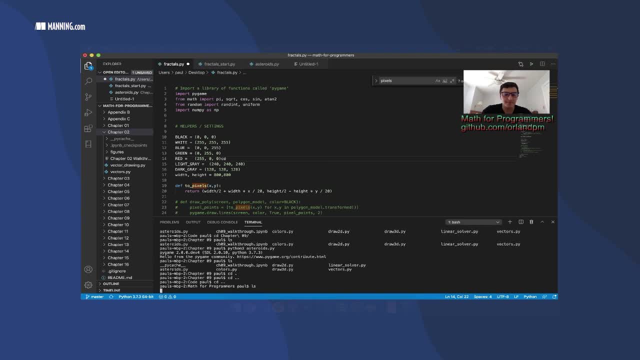 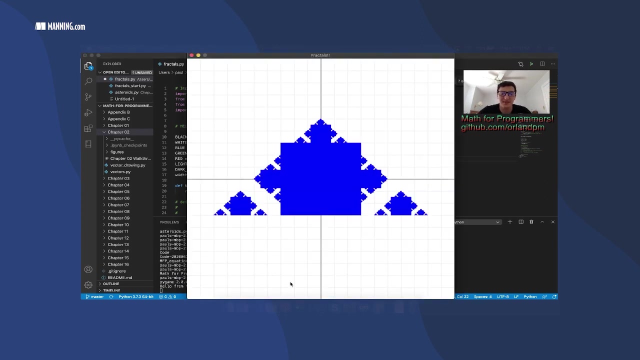 Let's see. So the example that I put together for today is: we'll make something that looks like this. So this, basically, you can see, it's kind of the same coordinate. It's kind of the same coordinate grid here as from the first example. 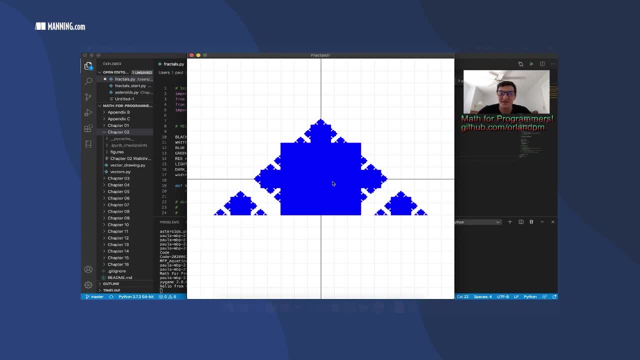 But I put together a fractal here, So it's a- this is a self similar geometric object. You can see that it's kind of like this square, the big square, And then next to it there are two little squares, And basically this pattern is repeated everywhere. 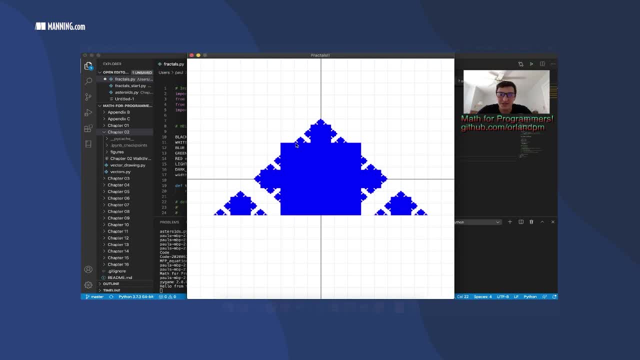 You see an edge now. So here's an edge of the original fractal And you see a big square and two little squares next to it. And then, on top of this little square, there's a big square and two little squares next to it. 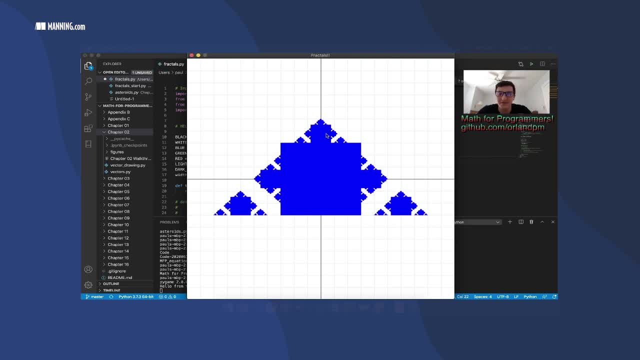 There's just one example. We can maybe do a couple of different examples, But the other thing that I wired up here is I just like the asteroid game I wired up So if you press different keys you can zoom in and see the fractal closer up. 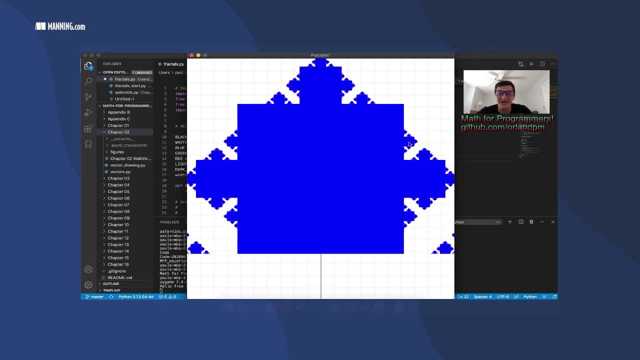 So you can actually see a little bit more detail as you zoom in here. Yeah, so that's the basic idea. I guess we'll get started now And I'll kind of just talk through, for the example, this example. I'll talk through how to write some of the code to make this work. 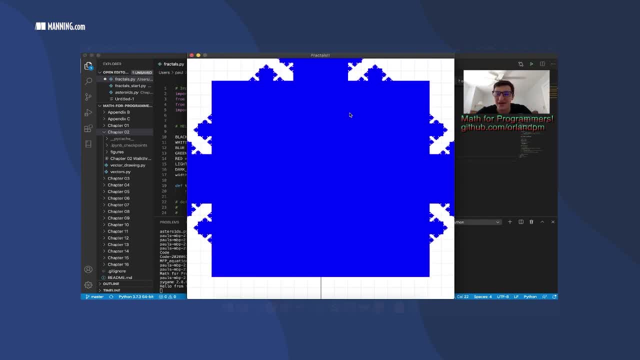 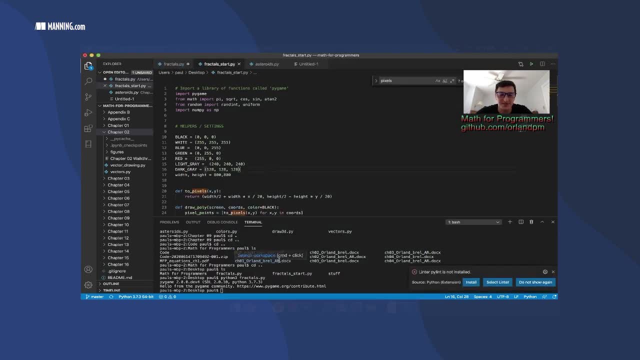 And then also some of the mathematical ideas that are behind the fractal or this fractal in particular, and then fractals in general. So to start basically, I put together this fresh version And let me make sure it's called fractals start. 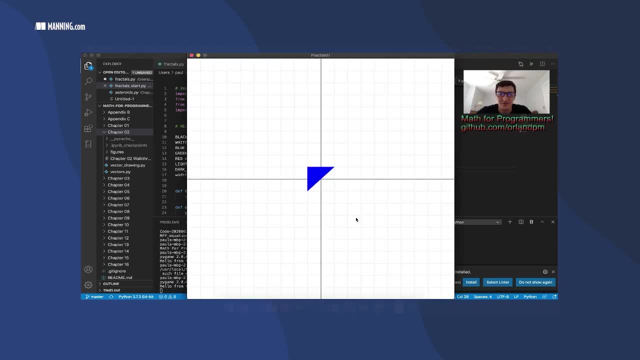 And let's see, It doesn't have much. So I wanted to make sure before I got started, that I had something going here. So here's just a graph. This is a single polygon, This is a triangle, obviously, And I wanted to make sure that I could draw this using the Python code. 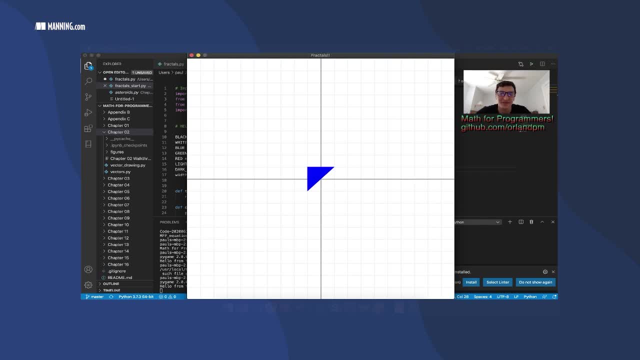 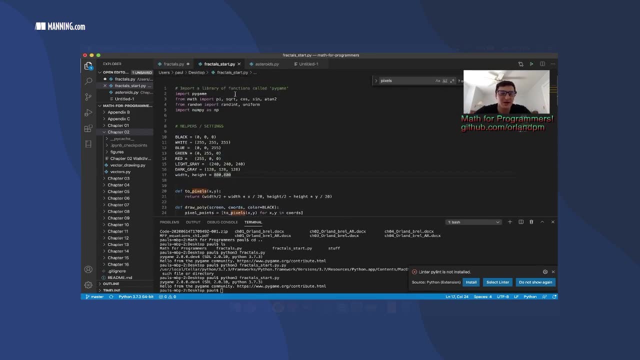 And so basically, we'll do everything else to get to a fractal, starting from this single polygon. So I'm not going to explain all of the code here. I'll give you a sense of the big things that are going on And, like I said, if you want to understand the code at a deeper level, a lot of this came from Chapter 9 of the book Math with Programmers. 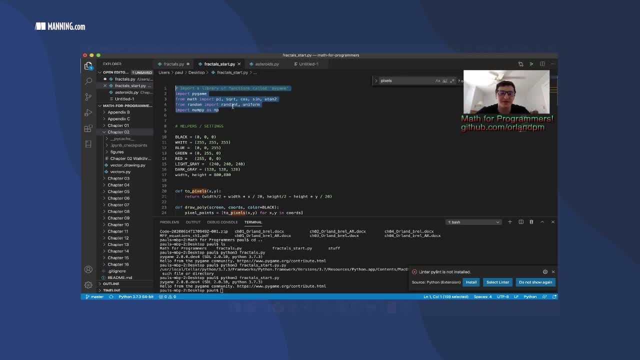 So you can find it online. There are a couple of libraries- Python libraries- that are imported here. There are a couple of colors and settings, So I set the width and the height of the game screen. I set the width and the height of the game screen to 800 pixels each to kind of make it big. 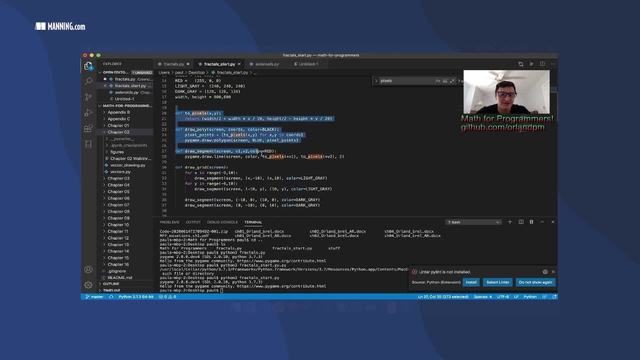 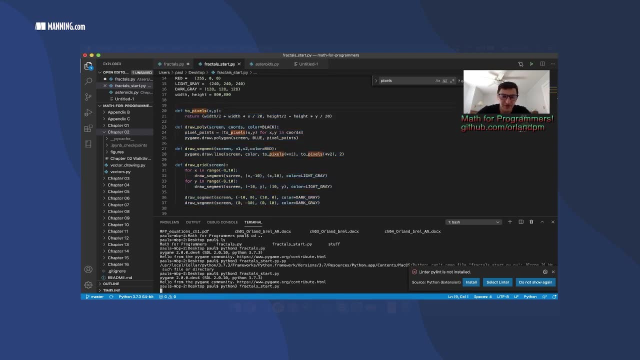 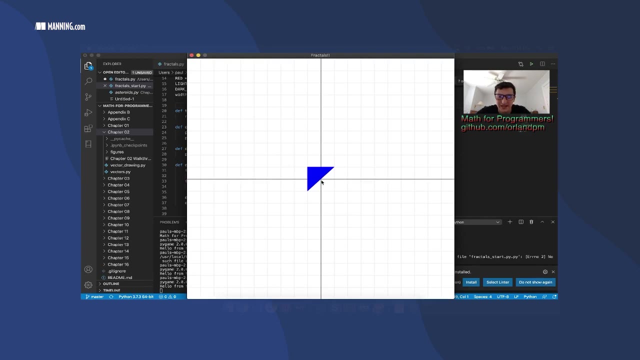 And then the next thing that are released in this code file- I think it's also in the code for Chapter 9, is there's a couple of helper functions. So when we're working with this, all of our computations will be done in this coordinate system, where this is like 0, 0. 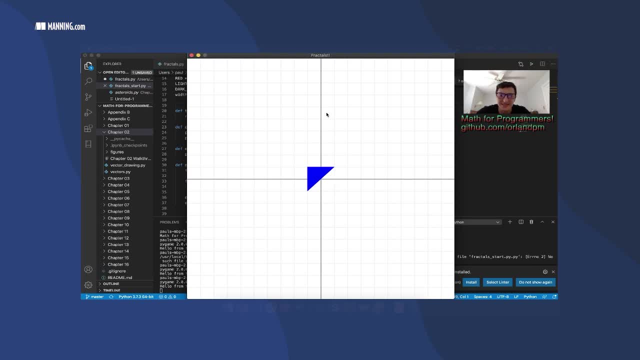 And this is one unit, And this is the x-axis And this is the y-axis, So you'll have one unit in the x-direction, two units in the x-direction, et cetera. So basically, your coordinates for a point are, however many, in the x-direction. 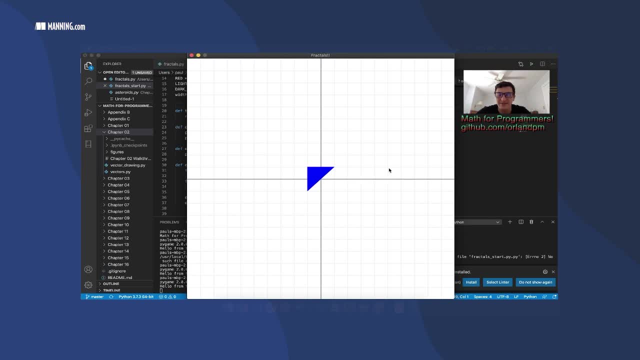 So maybe 1,, 2,, 3,, 4,, 5.. And then however many in the y-direction: 1,, 2,, 3.. So this is the 0.5, 3.. You probably remember this from a high school math class or something: how to find points in the coordinate plane. 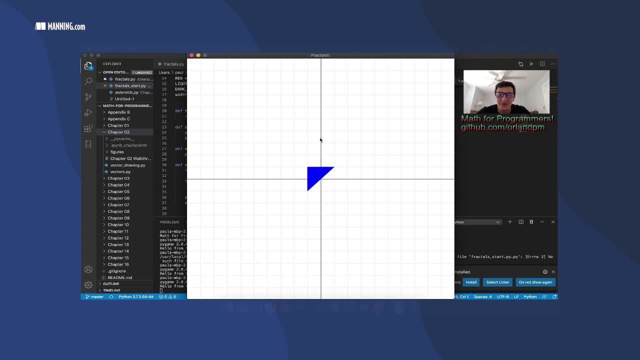 But if you don't, this is all covered in Chapter 2 of Math with Programmers. What I want to do is I want to think about geometry in this coordinate plane and then have it automatically convert everything to pixels for me. So that's what this helper function does. 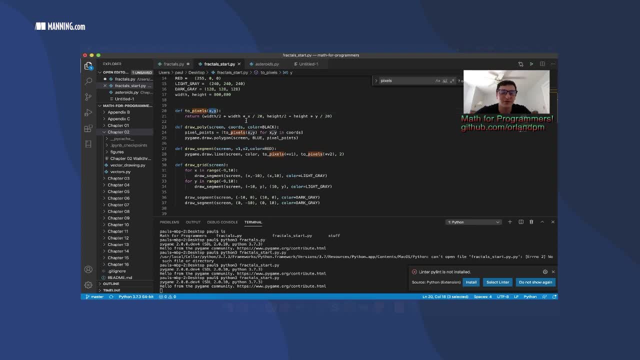 If I have an x and a y coordinate in this coordinate plane, then it basically does the math automatically in terms of the height and width to find the pixel values. So if you can draw a point at a certain pixel location, you can automate the process of drawing a polygon or drawing a line segment. 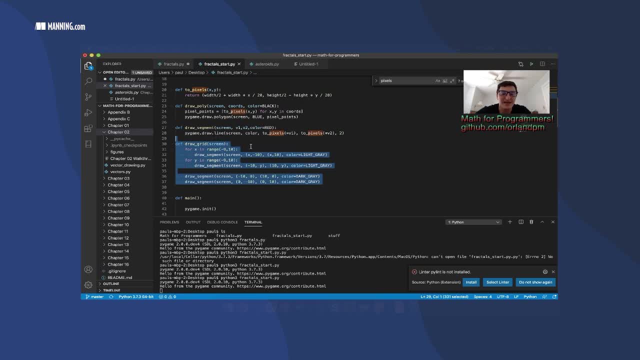 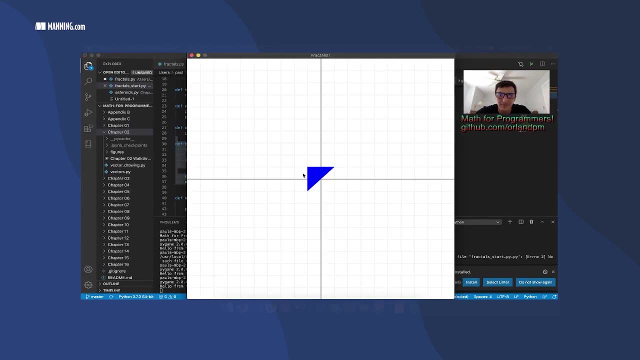 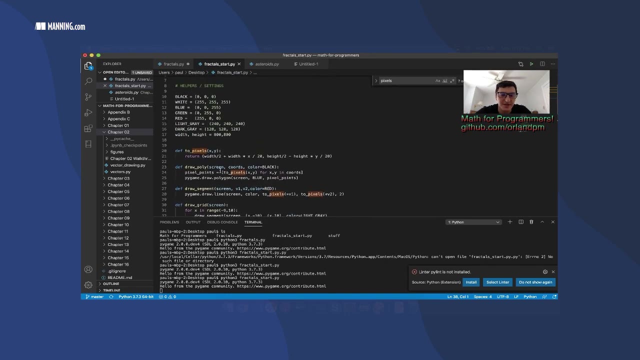 or actually this grid itself is kind of put in a helper function where it draws all of these vertical and horizontal lines to show me the coordinate axes, And I think that's all you really need to see for the helper functions. So then we get to the main function. 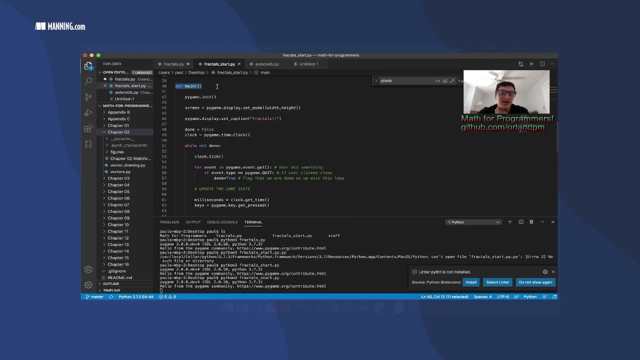 So this is the function that will be called when you actually start this Python script, And this is mostly using a Python library called Pygame. Pygame is a framework designed to help you create an interactive game simply in the Python programming language, So it basically gives me tools to create that screen. you saw. 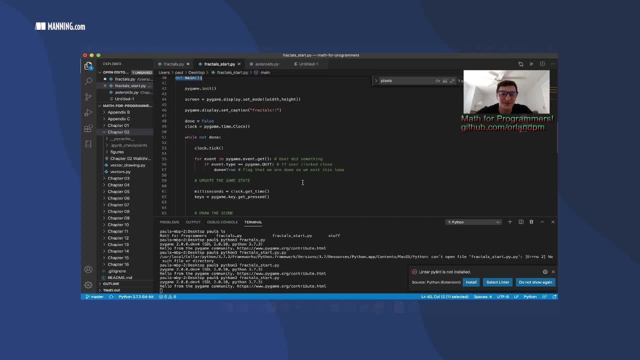 make it interactive, have it refresh on a recurring basis so we can animate it. And a lot of that is explained in the appendices of Math for Programmers, because we use Pygame in a couple of chapters. So the main part of the Pygame program is this thing called a game loop. 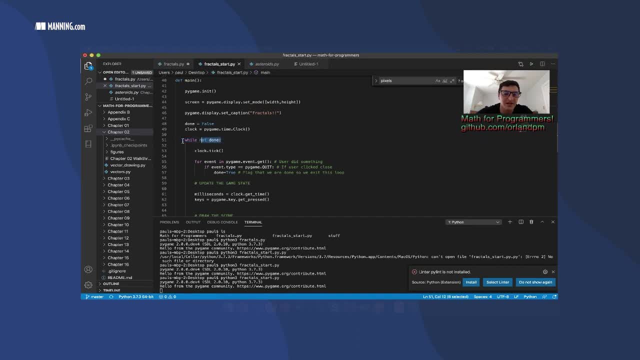 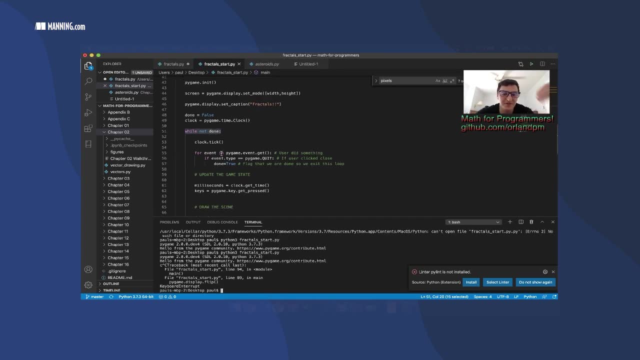 So it's while not done, basically while we haven't said to shut down the screen, it's going to do a bunch of things over and over again, And the first one is it updates the clock. So there's a clock in the background and then while 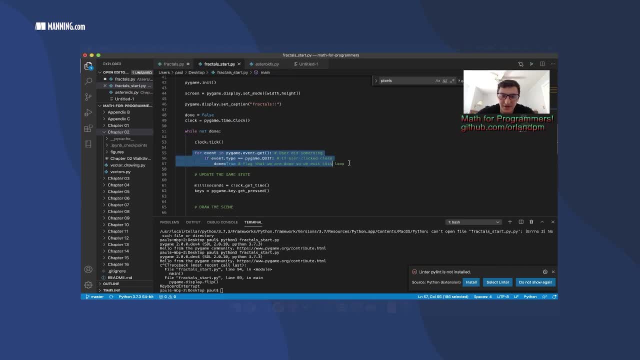 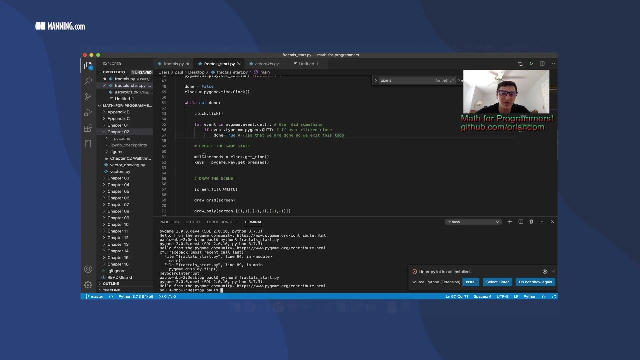 let's see. I guess if you press the X button on that screen, if you press this X button, it exits and it breaks this while loop, But otherwise it doesn't set this done to true and it keeps looping through this, So it knows the number of milliseconds that have elapsed since the last frame. 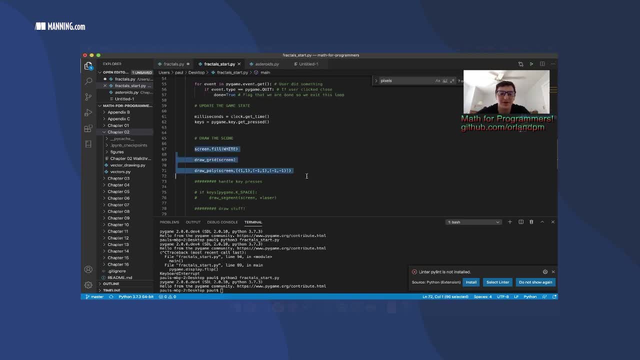 And then it basically does some drawing in every frame, kind of like you can think of frames of a movie, And every time it starts it sort of goes through this while loop. It'll draw a new frame, And that's how you saw in the first fractal I showed you. 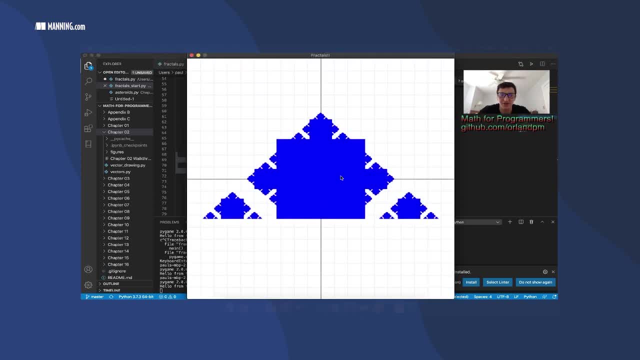 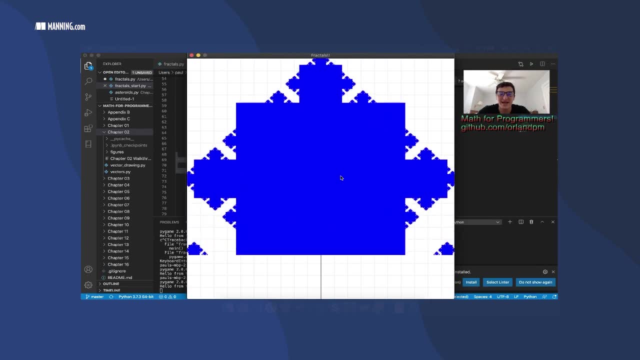 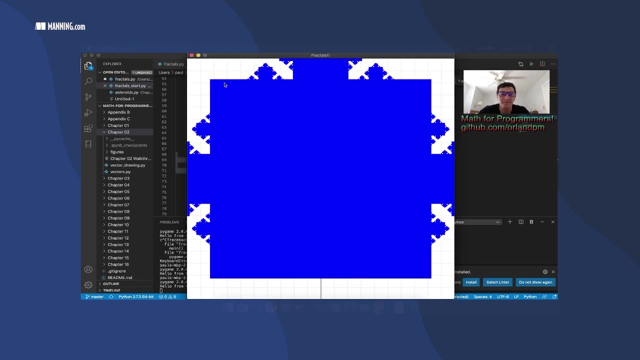 Let's see, And the first fractal I showed you that actually animates. So this is every time I hold down a key on my keyboard, it's animating, it's drawing a new version of the fractal in every frame And that's why you see it getting bigger. 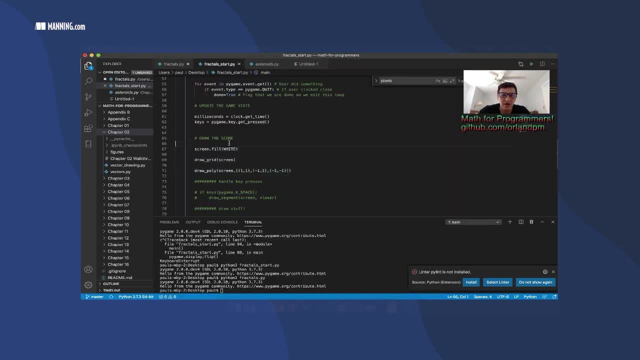 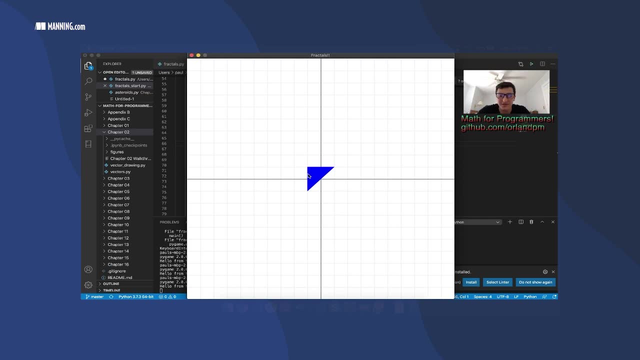 It's just drawing it over and over again. Okay, So now I'm back in this fractal start file where I've only got one polygon, And what we'll do is we will draw a similar kind of fractal, this self-similar, complex geometric pattern, starting from here. 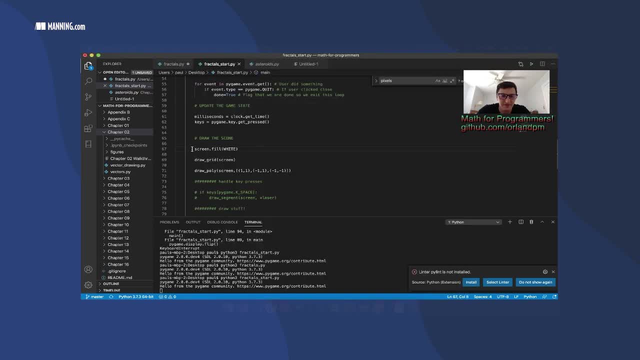 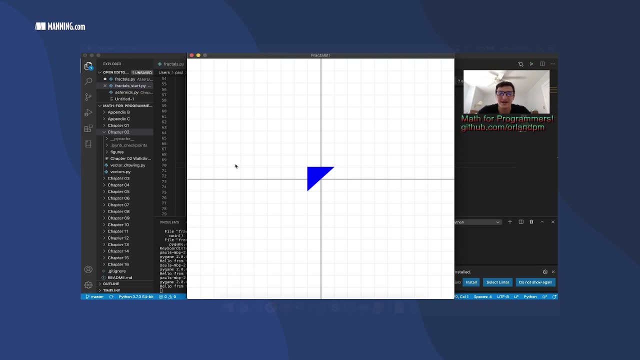 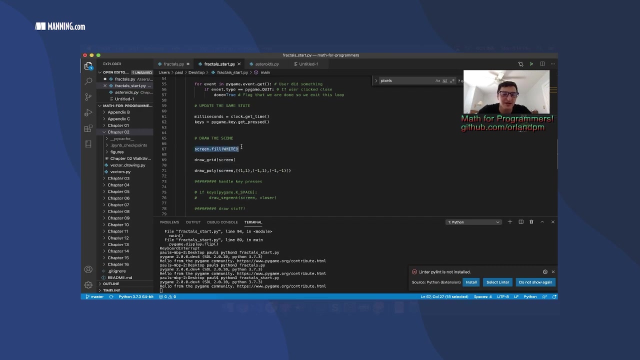 And you can see. there's a couple of lines that are drawn every frame of this animation. You don't see it moving, but it is an animation. This is being redrawn some number of times, every second, to get this triangle showing up, The first thing that happens in every loop and in every frame. 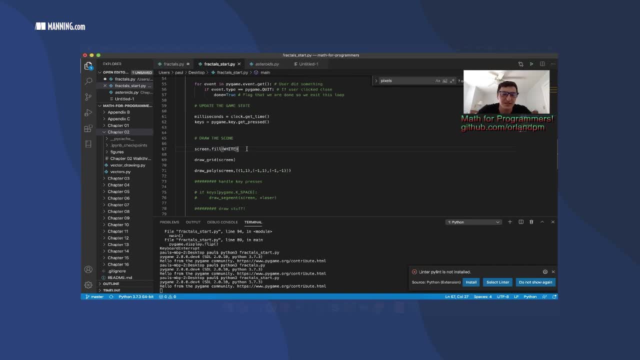 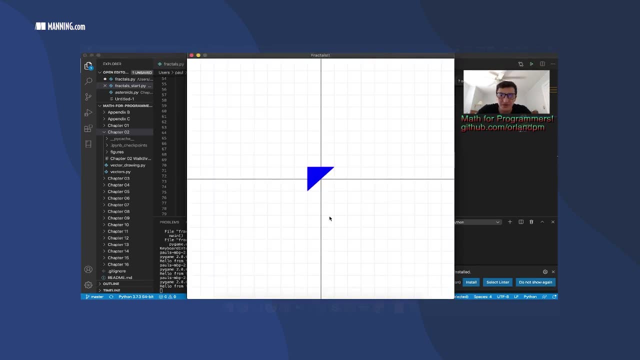 is that the screen is filled with white. So we basically blank out everything that's on the screen And then this grid is drawn, So you see the horizontal and vertical grid lines. So that's what drawGrid does. And then you get drawPoly draws a polygon. 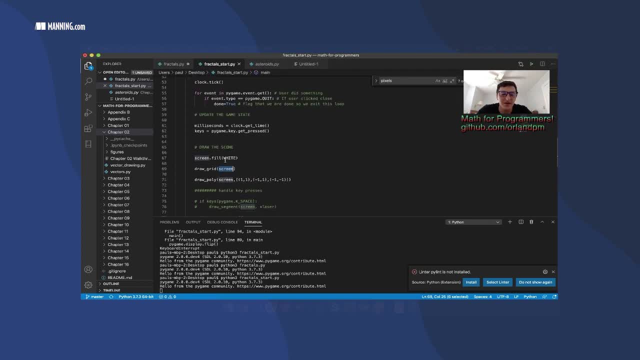 And there's this screen variable that represents that window. So drawPolygon is this wrapper that takes in the screen And then it takes in a list of coordinates, which are the vertices of the polygon. What you've got here are 1, 1.. 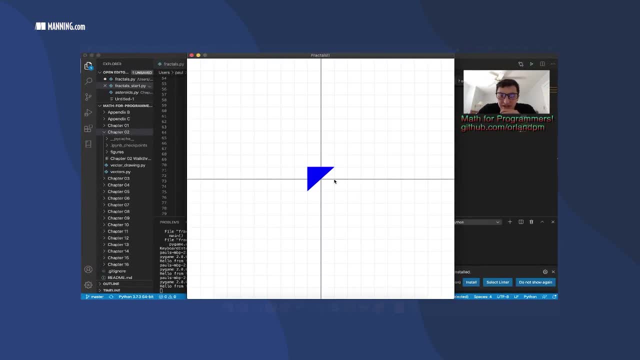 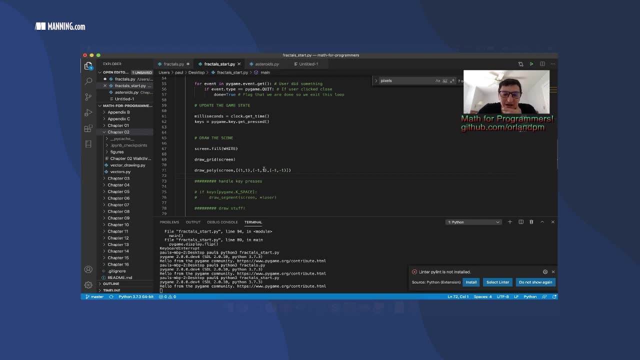 And that is: let's see: 1, 1 will be 1 in the x-direction, 1 in the y-direction. so that's this vertex. And then you've got negative 1, 1.. And that is: let's see negative 1, 1 will be this vertex. 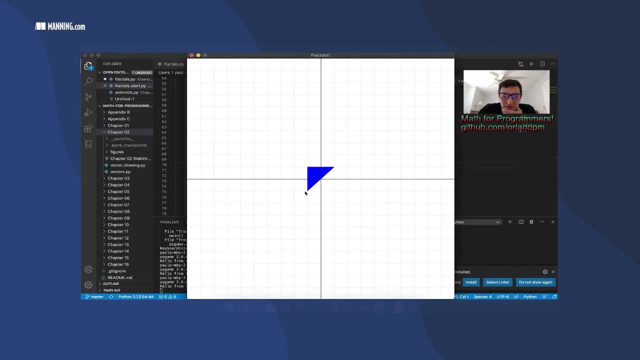 And then the last one will be negative 1, negative 1, which is this guy here? negative 1 in the x-direction and then negative 1 in the y-direction. So those three together give us our triangle, And this drawPoly function kind of knows how to fill that in. 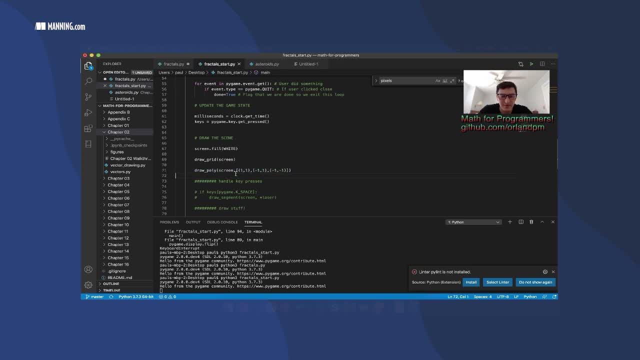 So I guess, as a first example, maybe I'll try making this a little bit bigger. We've got a lot of screen space to work with. So if you change all of the numbers and make them bigger, then everything will get bigger by the corresponding factor. 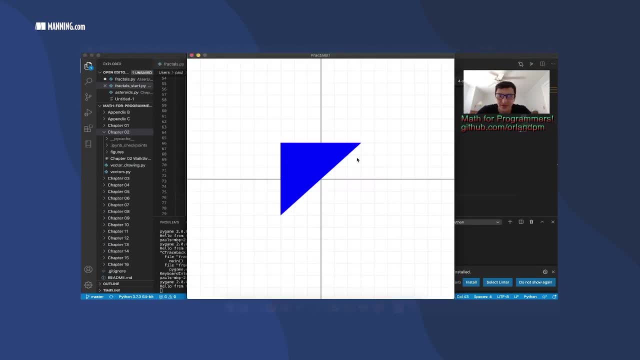 Let's take a look and see what this does. We'll have to restart the Python script And you can see the triangle got bigger. So now it's like 3, 3, negative 3, 3, and negative, 3, negative, 3.. 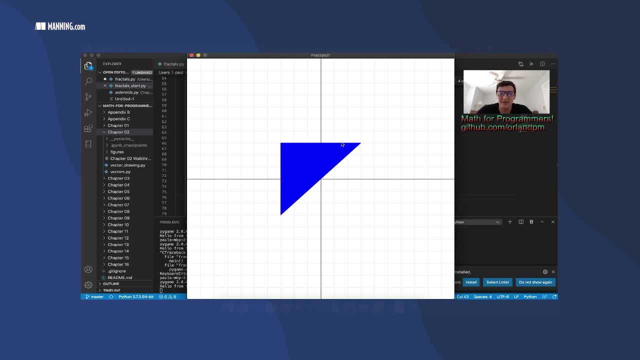 OK, so that's a good start. Maybe we can- actually I didn't plan on doing this- we can try doing a triangle-based fractal in this demo and see where that gets us, instead of the other example that I showed you, which was based on kind of a self-similar pattern of squares.